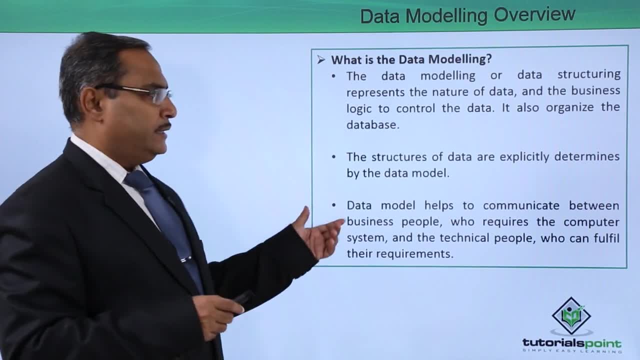 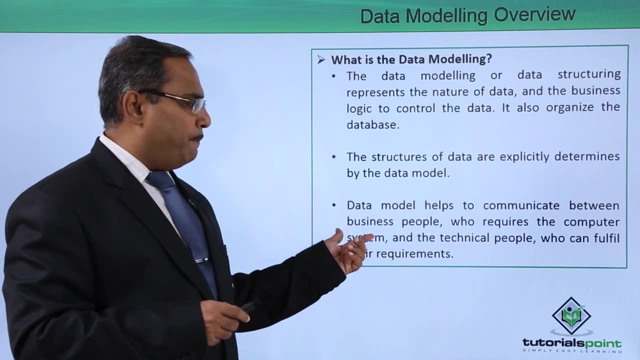 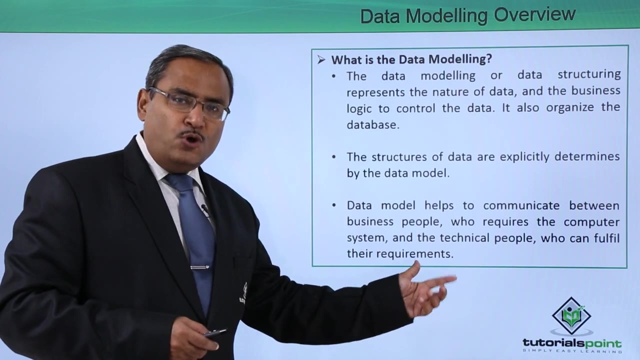 will actually decide what will be the structure of the data, And that will be decided explicitly. Data model helps to communicate between the business people who requires a solution, So who requires a computer system- And the technical people who is going to implement the respective solution and will provide the 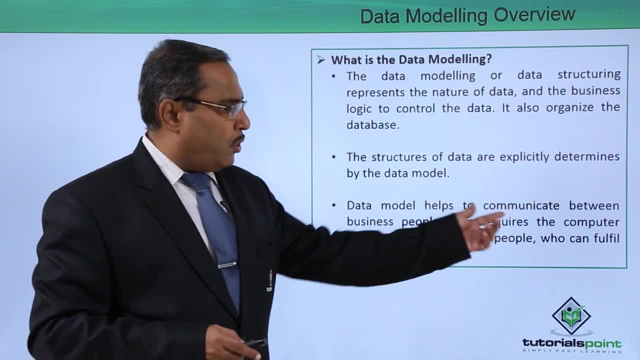 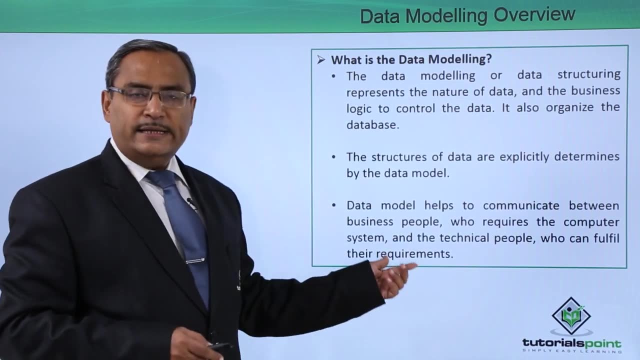 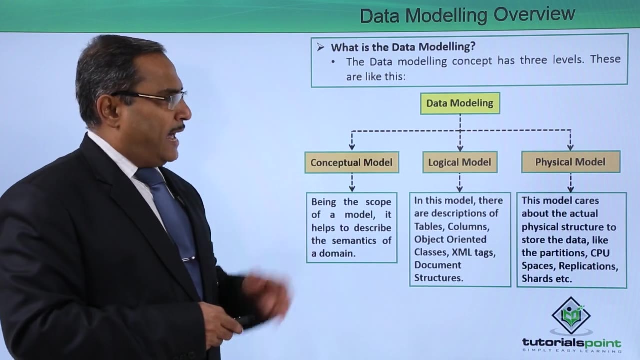 service to these business people. So the data model helps to communicate between the business people who requires a computer system and the technical people who can fulfill their requirements. So that is why data modeling is so important. So the data modeling concept has three levels. 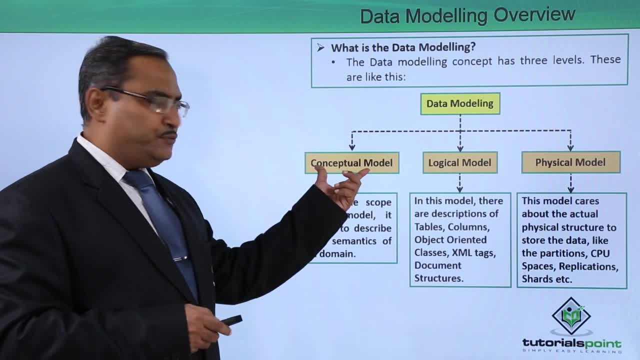 And these three levels are like this: First one is the conceptual model, Next one is the logical model, Next one is the conceptual model, Next one is the logical model, Next one is the logical model And the last one is the physical model. Now, what is the conceptual model? 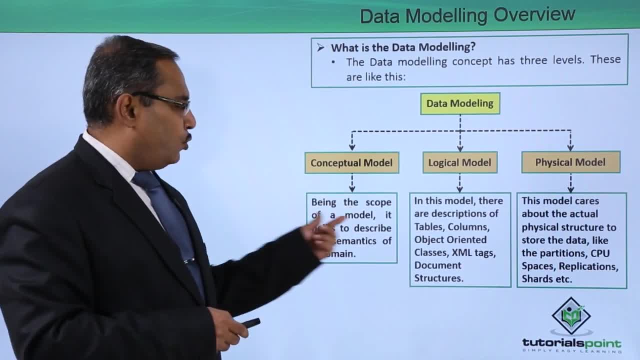 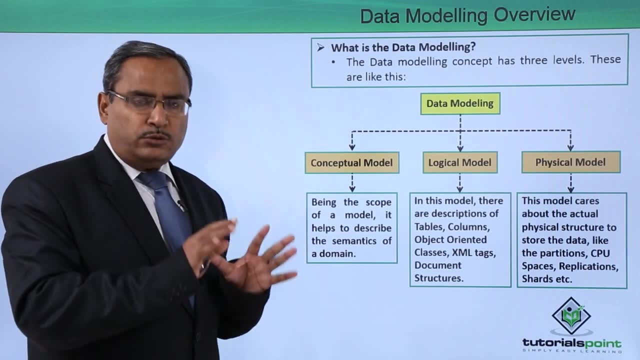 We have written a very summary for it. So, being the scope of a model, it helps to describe the semantics of the domain. So it is not actually related that how the data will be stored, what will be the respective data types. It is not dealing with that. It is dealing 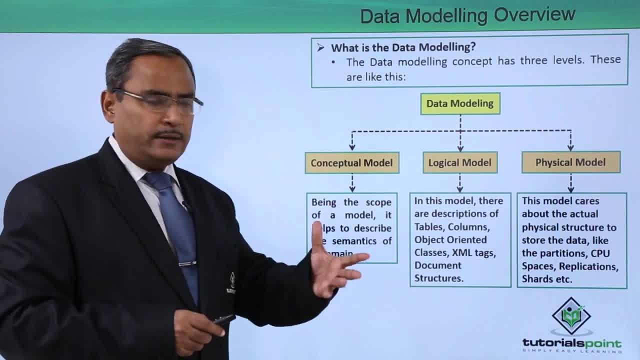 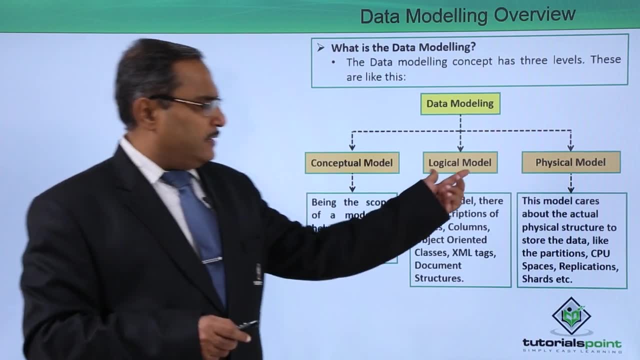 with the semantics of the domain. Semantic means meaning So, being the scope of a model, it helps to describe the semantics of context. Now let us go for the next phase, that is, the logical model. In this model, there are: 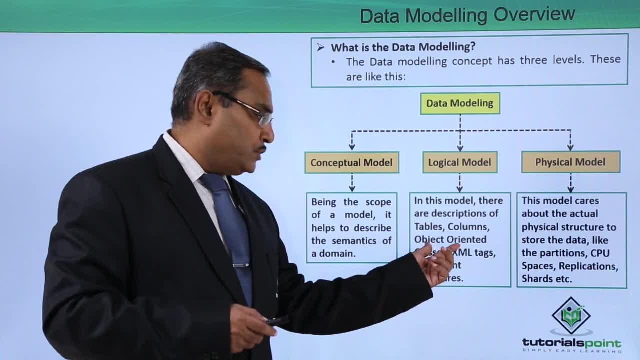 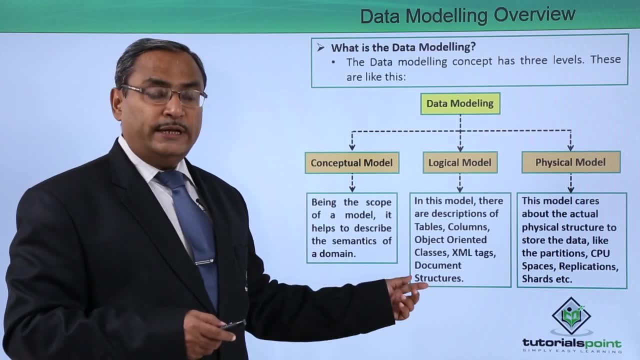 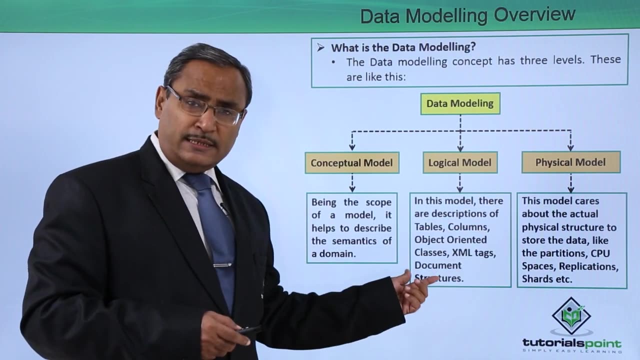 descriptions of tables, columns, object-oriented classes, XML tags, document structures and so on. So here we are having all the detailed descriptions. So this model: there are descriptions for tables, columns, object-oriented classes, XML tags and document structures and so on. 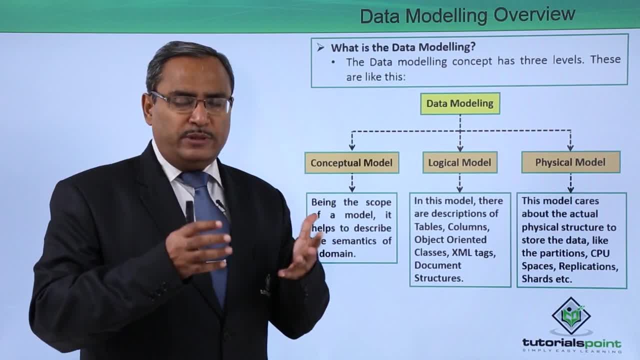 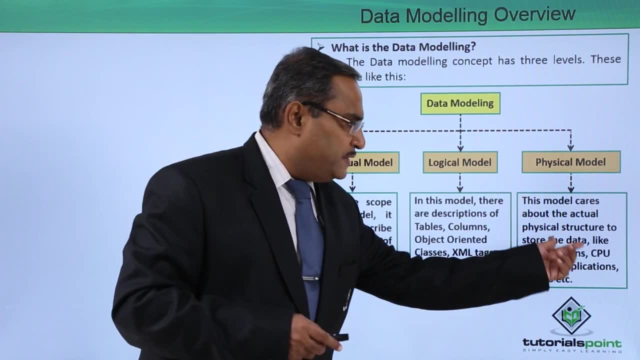 Next one is a physical model, And this particular model is actually dealing with the fact that how the data will be stored into shards and in other way. So this model cares about the actual physical structure to store our data And, like the partitions, CPU spaces. 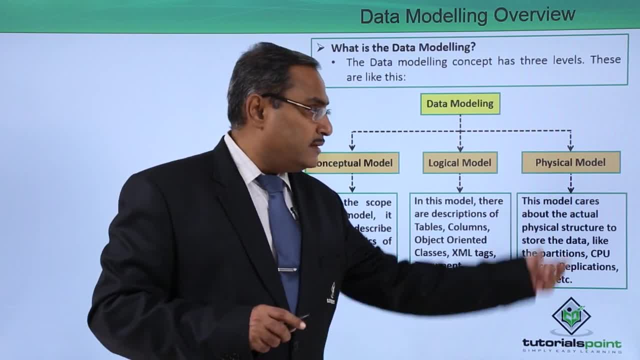 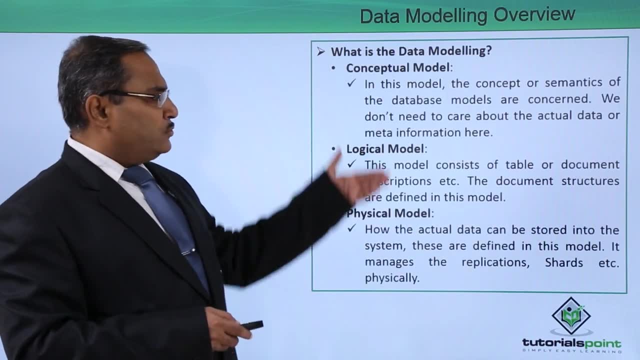 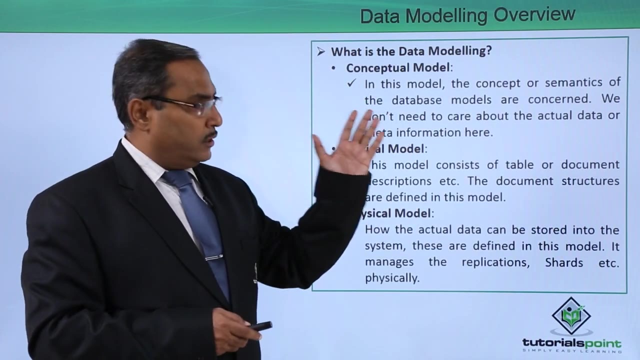 replications, shards, etc. So this is known as the physical model. It is dealing with the fact that how the data will be stored. So let us go for a quick summary. So, conceptual model, As we have mentioned that the data is stored in six contextual frames And in: